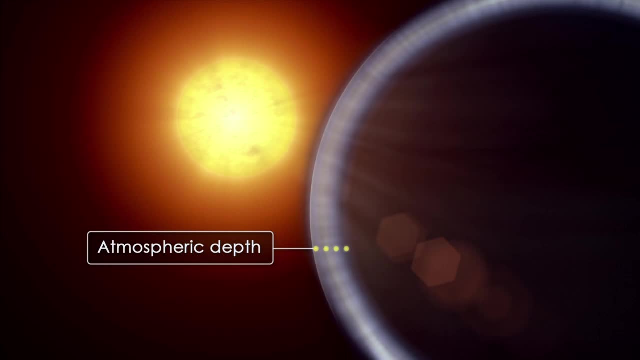 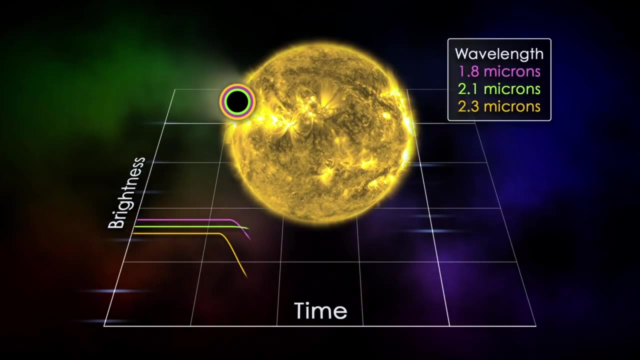 Organic molecules are the building blocks of life. They include amino acids, lipids, carbohydrates and nucleic acids. Organic molecules can be detected in the atmospheres of exoplanets using a technique called transit spectroscopy. Spectroscopy involves splittings. 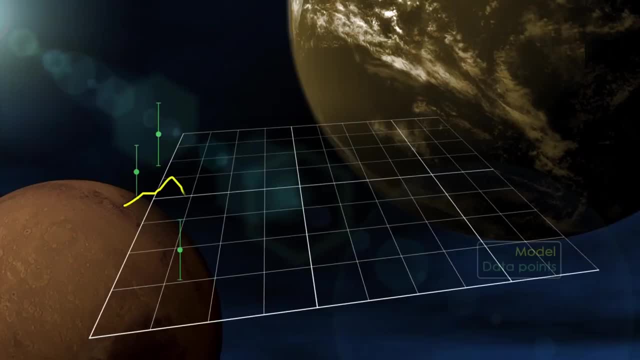 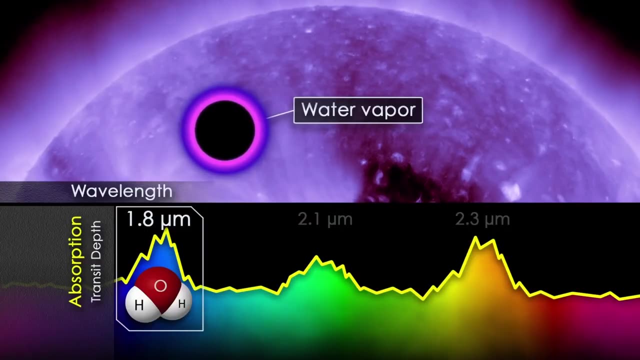 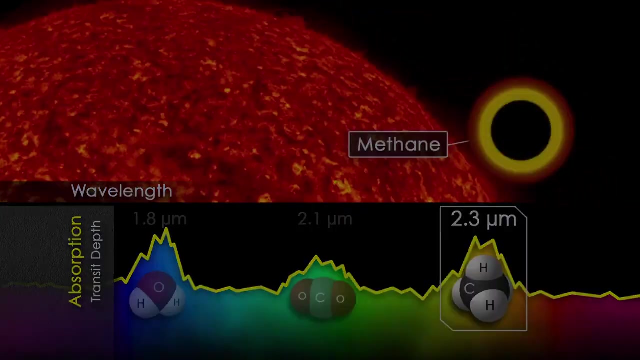 which allows the exoplanet to send light into its component wavelengths. Organic molecules absorb light at specific wavelengths, so by looking for dips in the spectrum of an exoplanet, scientists can identify the presence of organic molecules. JWST is currently the best instrument we have that can detect biosignatures in this way. 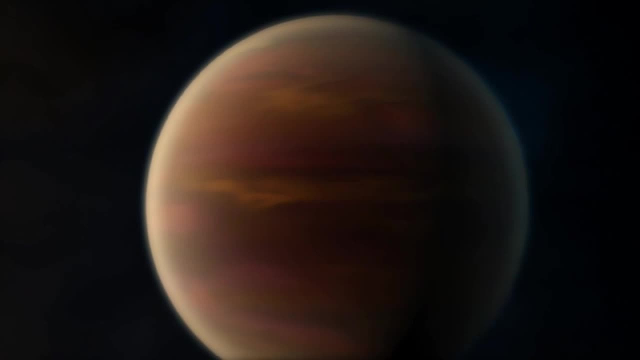 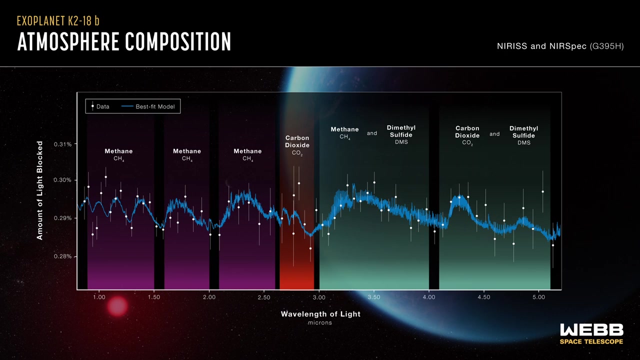 It looks at absorbed starlight that has passed through the exoplanet's atmosphere to see what elements were absorbed. Just recently, it reported the possibility of the organic molecule dimethyl sulfide in the planet K2-18b, a compound that on Earth, is produced primarily by phytoplankton. 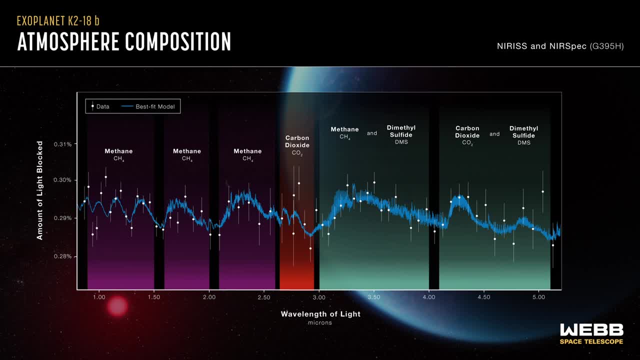 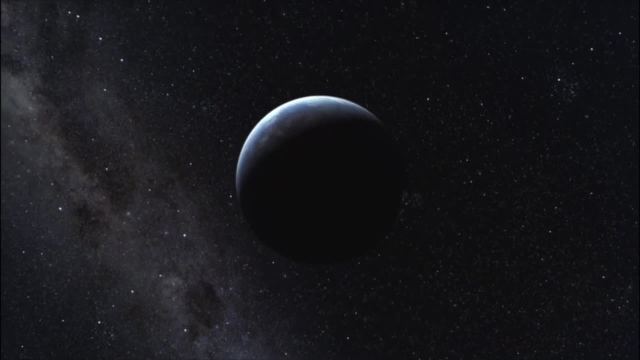 which are microscopic organisms that live in the ocean. Dimethyl sulfide can also be produced by some other biological processes, but it is not known to be produced by anything other than life. Dimethyl sulfide is a gas, so it can be detected in the atmospheres of exoplanets using spectroscopy. 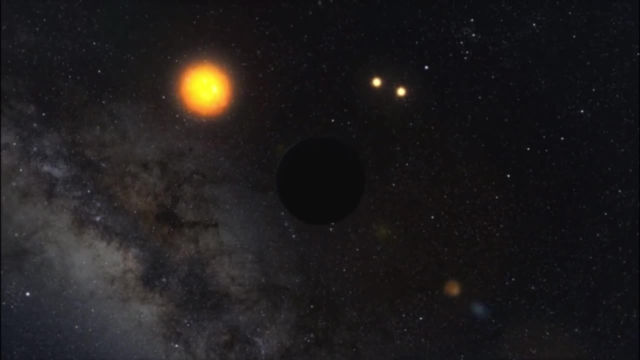 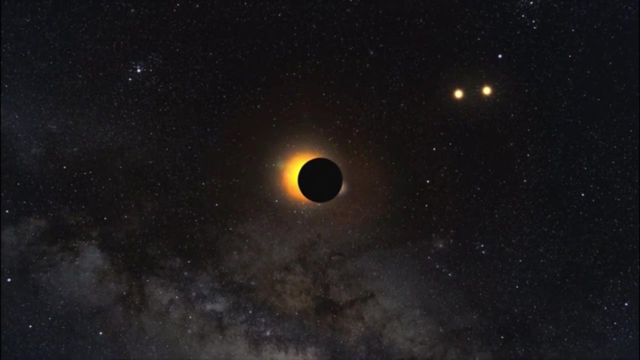 It is also relatively stable in the atmosphere, so it can accumulate to detectable levels. All this makes dimethyl sulfide an ideal biosignature gas. It's important to note that the detection of a single biosignature is not definitive evidence of life. 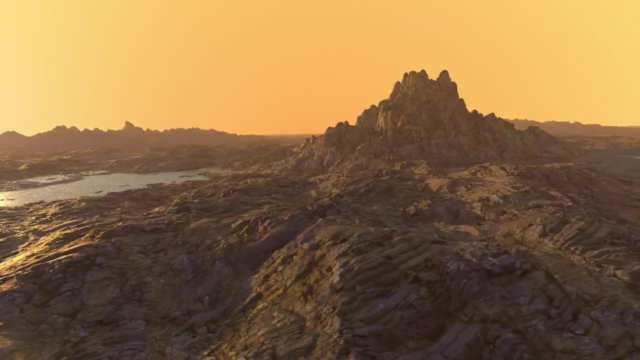 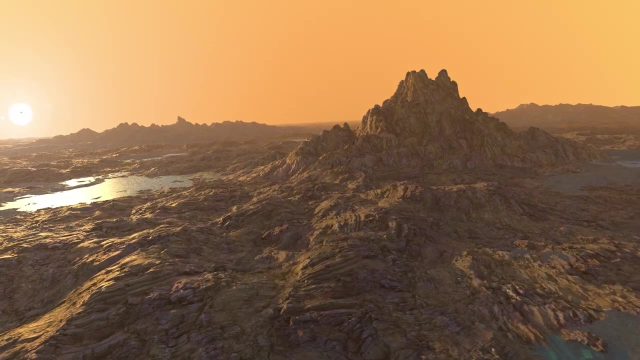 However, the presence of multiple biosignatures in the same place would be very strong evidence. Additionally, if a biosignature is detected in a place where it is unlikely to be produced by biological processes, such as say, in a Martian meteorite. 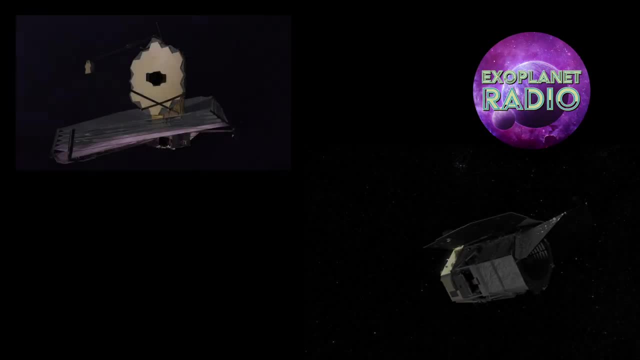 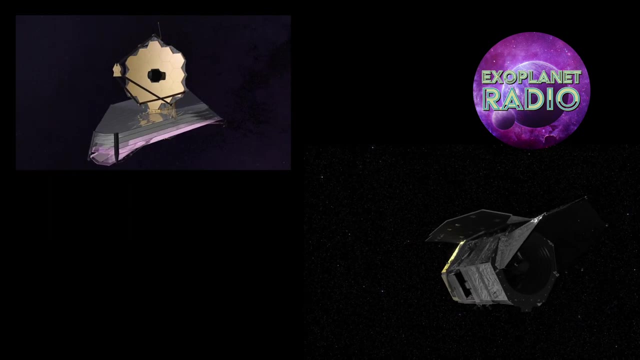 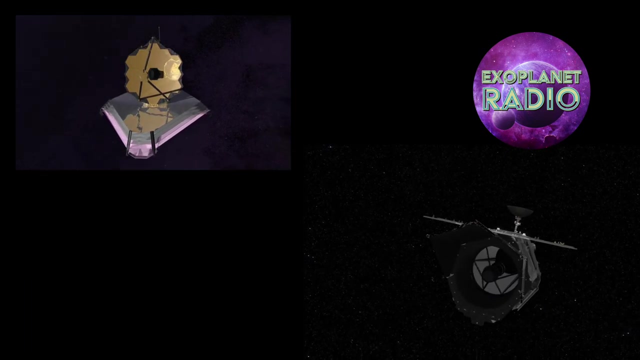 then it is more likely to be a sign of life. The James Webb Space Telescope and the future Habitable Worlds Observatory are two powerful tools that we have to search for life on other planets. Imagine the day when we discover signs of life beyond Earth. 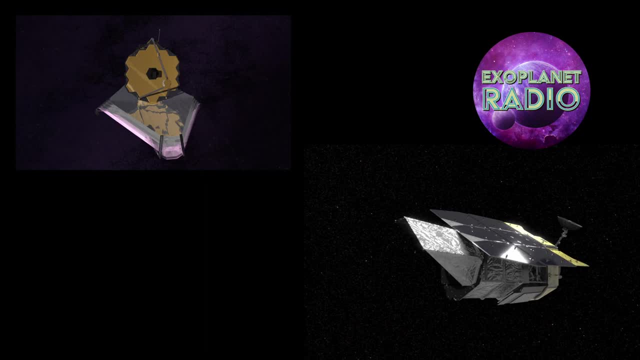 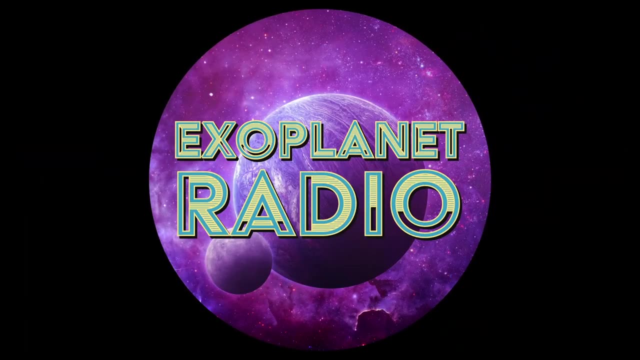 It would be a watershed moment in human history, one that would change our understanding of our place in the universe forever. Exoplanet Radio is produced by Deep Astronomy, The music is by Geodesium and available at Loch Ness Productionscom. Get all episodes from exoplanetradiocom. or anywhere you get podcasts. 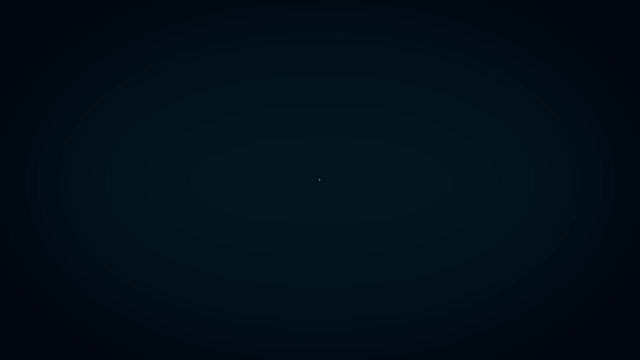 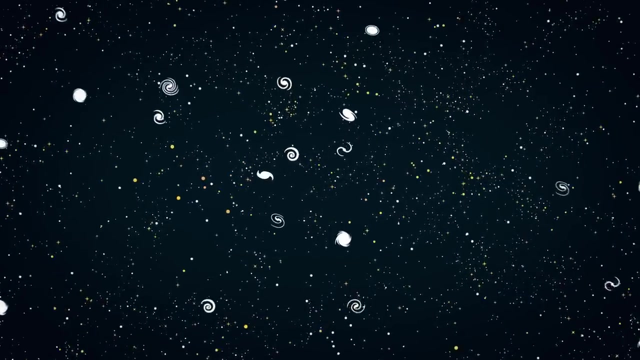 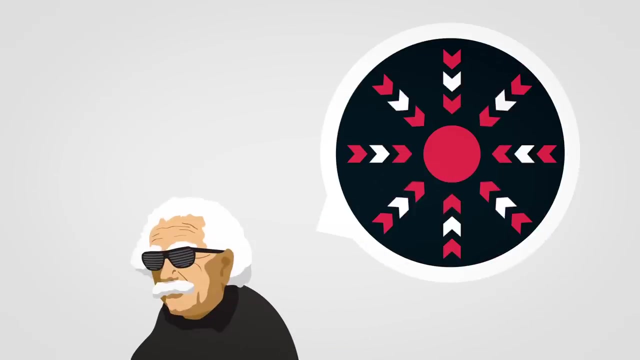 The beginning of everything, the Big Bang, The idea that the universe was suddenly born and is not infinite. Up to the middle of the 20th century, most scientists thought of the universe as infinite and ageless, Until Einstein's theory of relativity gave us a better understanding of gravity and Edwin Hubble 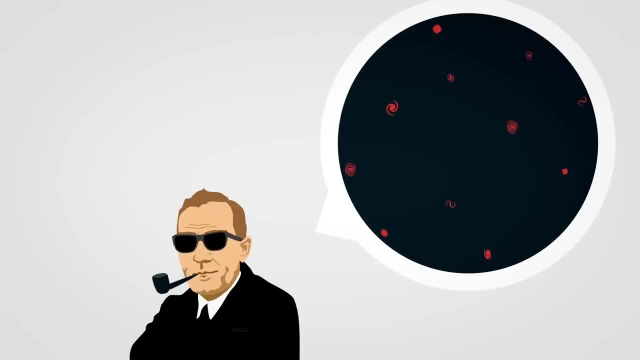 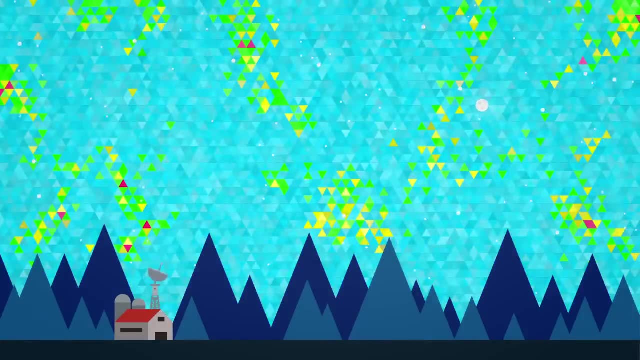 discovered that galaxies are moving apart from one another in a way that fits previous predictions. In 1964, by accident, cosmic background radiation was discovered, a relic of the early universe which, together with other observational evidence, made the Big Bang the accepted theory in science. Since then, improved technology like the Hubble telescope, 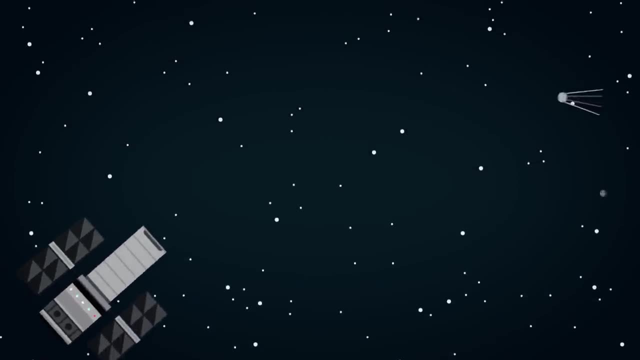 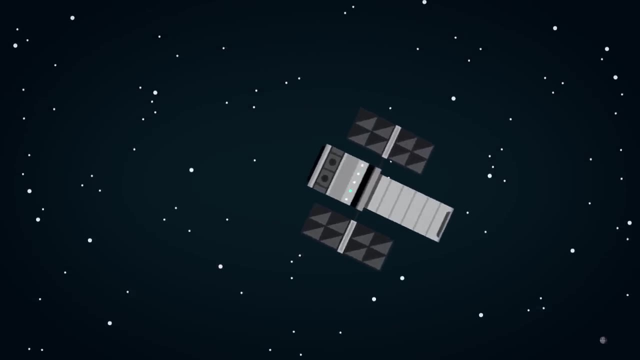 has given us a pretty good picture of the Big Bang and the structure of the cosmos. Recent observations even seem to suggest that the expansion of the universe is accelerating. But how did this Big Bang work? How can something come from nothing? Let's explore what we know. 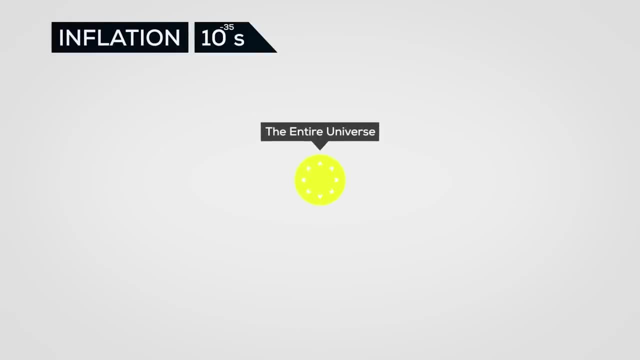 We can ignore the beginning part for now. First of all, the Big Bang was not an explosion. It was all space stretching everywhere all at once. The universe started very, very, very small and quickly expanded to the size of a football. 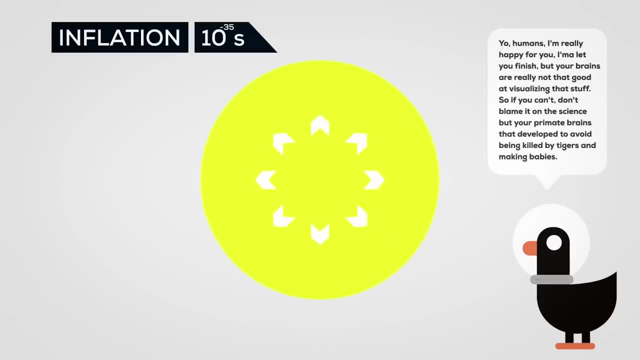 The Earth was not expanding into anything. Space was just expanding into itself. The universe cannot expand into anything. Finally, because the universe has no borders, some kind ofria or 97.8 gigahertz become completely覚. There is no outside of the universe. There is, by definition, no outside the 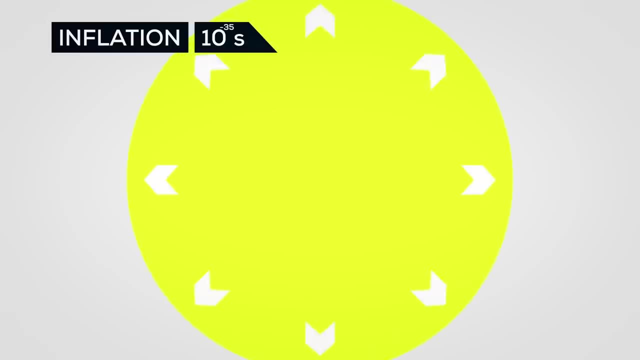 universe. The universe is all there is. It is still the Indigenous Universe. In this hot, dense and shadowy environment, energy manifested itself in particles that existed only for the tiniest glimpses of time. From gluons, pairs of quarks were created, which destroyed one.